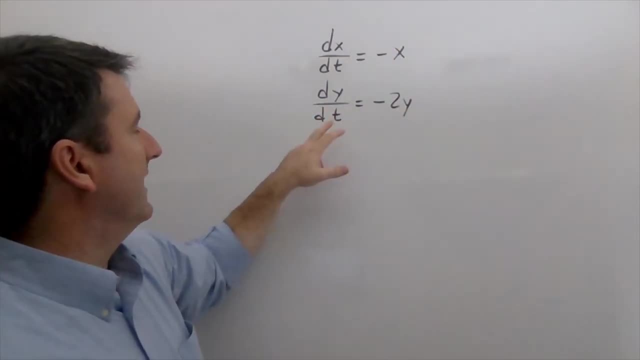 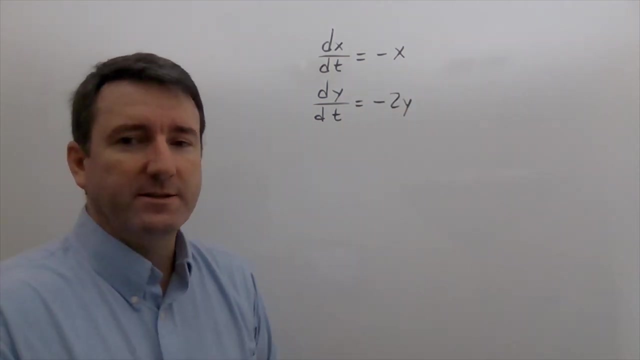 to negative x, no t here on the right side. Again here in this second equation, dy dt equals negative 2y, no t over there. So this is an autonomous system of equations. We're going to first find the critical points for this. 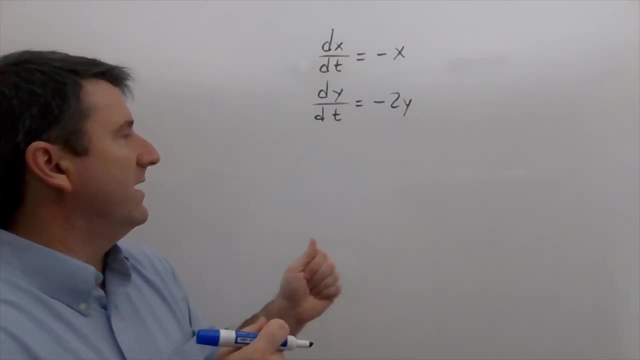 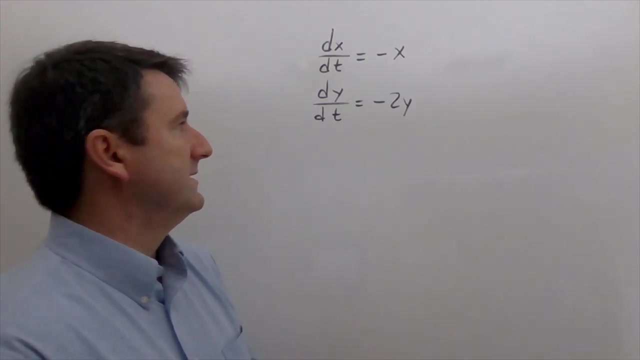 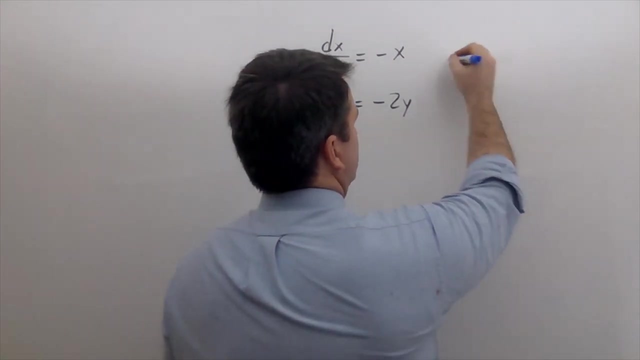 Now a critical point. by a critical point we mean a point where each of these functions, here these functions of t, are equal to zero. So here this negative x be equal to zero. So let's just set that equal to zero, Set both of these equal to zero, And then solve. 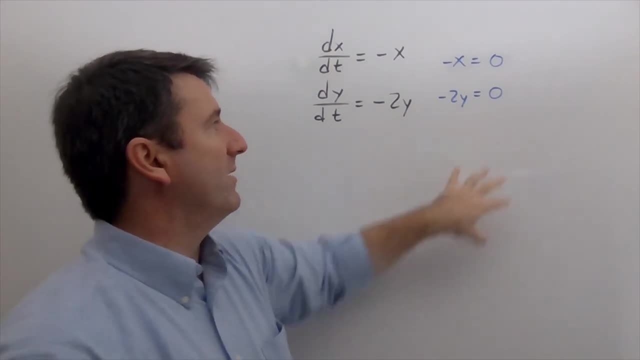 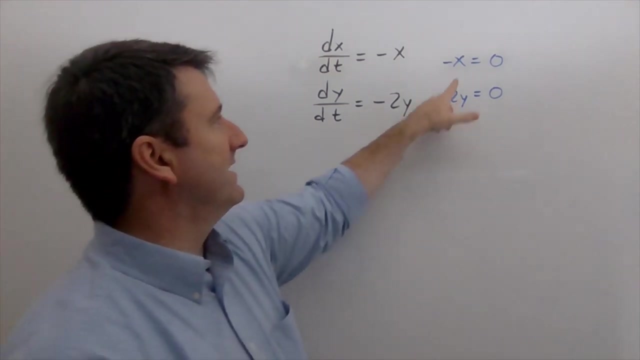 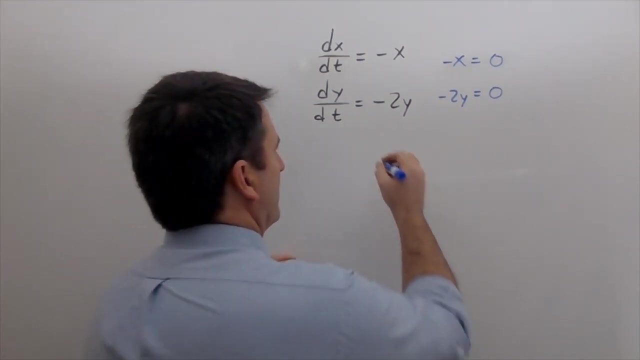 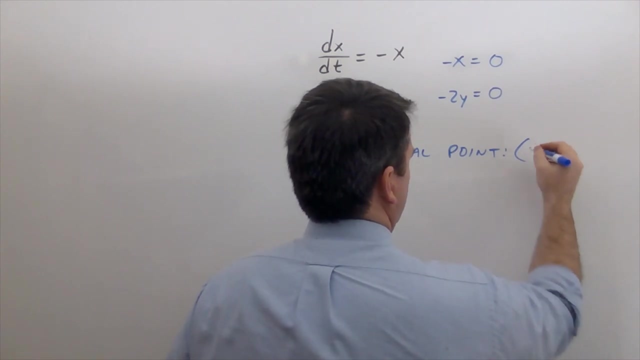 that system of equations to determine at what points are both of these equal to zero. Well, we can see that the only place where both of these are going to be equal to zero is if both x and y are equal to zero. So our critical point is going to be at the origin. 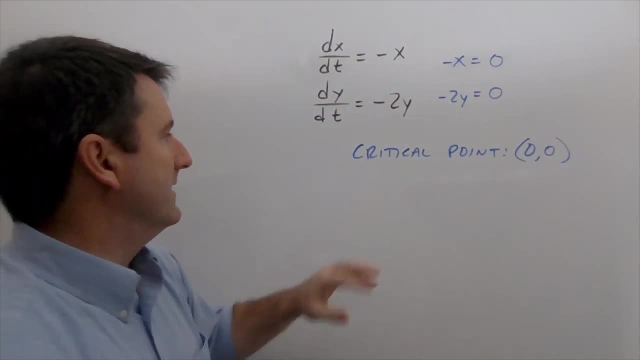 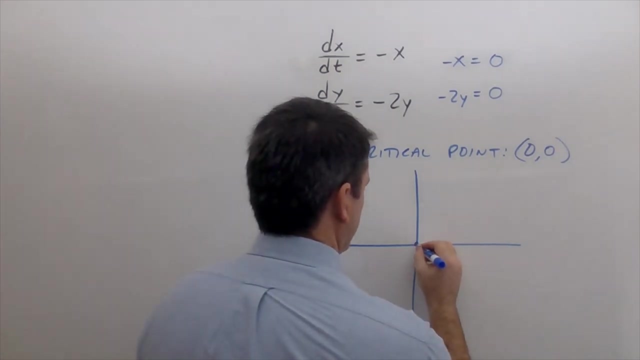 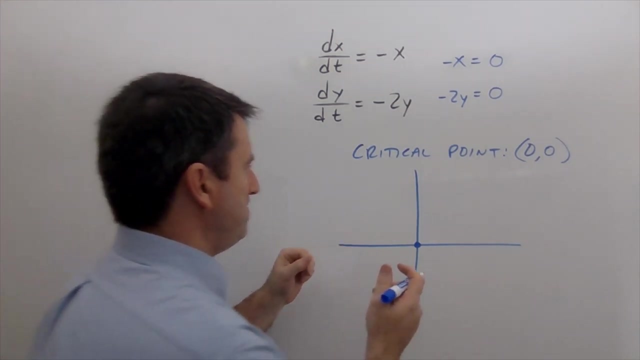 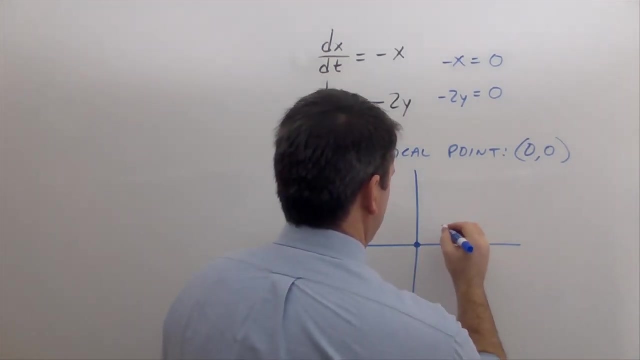 at Alright. so now let's graph what happens around that critical point. So here's our critical point And let's take some points near that critical point and draw the trajectories at those various points. So here let's take the point and the point and we'll go down here to 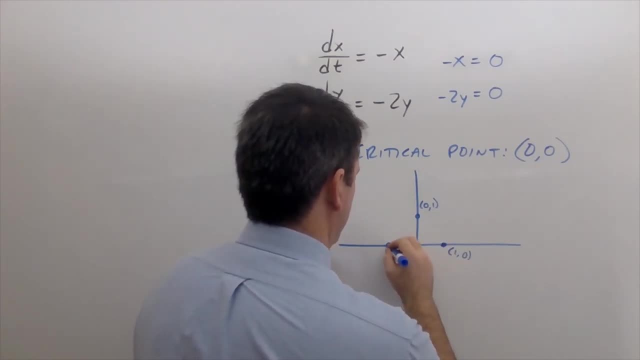 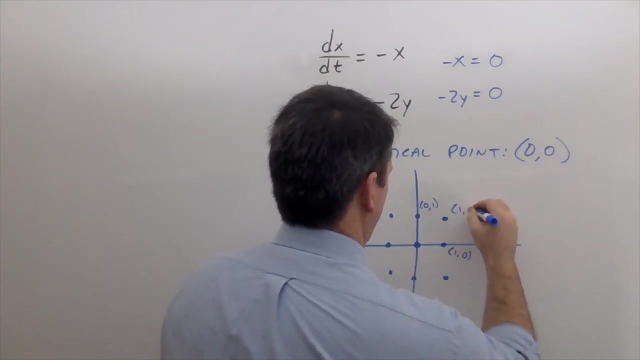 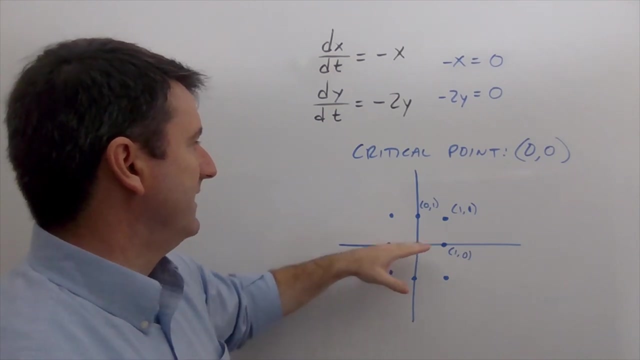 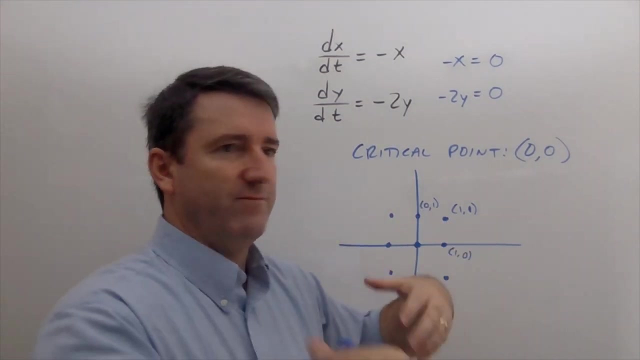 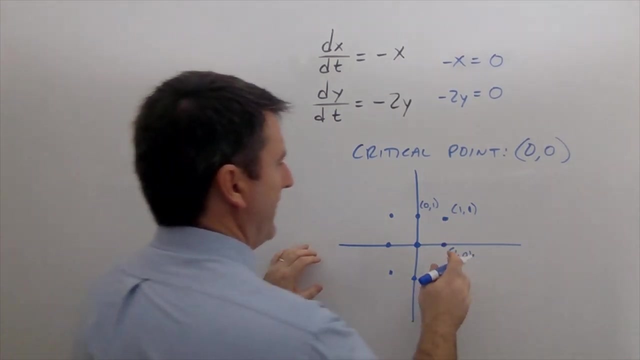 negative or zero. negative one, negative, one, zero, And then also these corner points here at Alright. so what I want to do is find the slope at each of those points and then what direction the solution is flowing. Alright, so at the point, let's start here at If x is one and y is zero, if we plug that in, 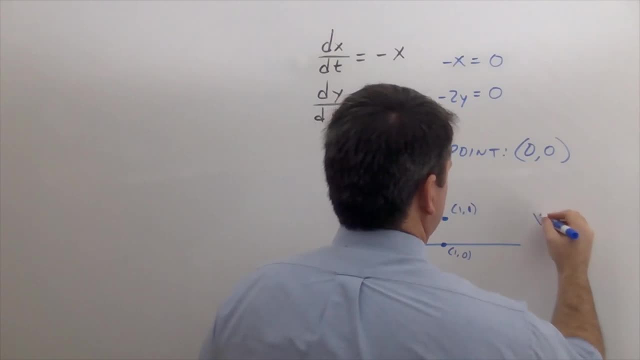 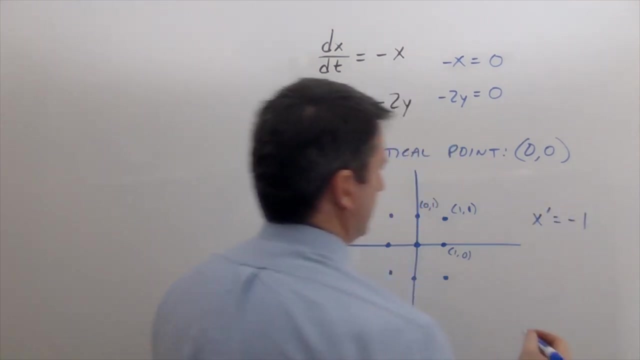 up here. we're going to get that the change in x- x prime is going to be equal to negative one, And then the change in y. if y is zero, that the change in y is so going to be zero, And so then the slope is going to be the change in y over the change in x, which 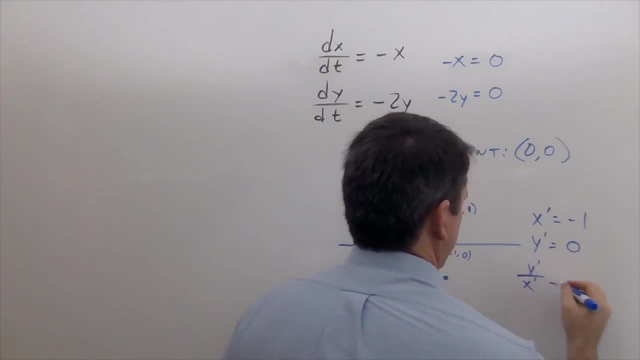 in this case, is going to equal to the slope of This. here is going to be the slope of x prime And itazuster justamente p, and then the slope is zero and that's how we get the split of x and we plug that in up here, we get that x prime and that's how we bring. us to the Olá interherмотриate, So negatively divided things. So then if x and y and y change, then that's in 참ottitalism, So that'sектор is equal to negative one, Mutually among all these. 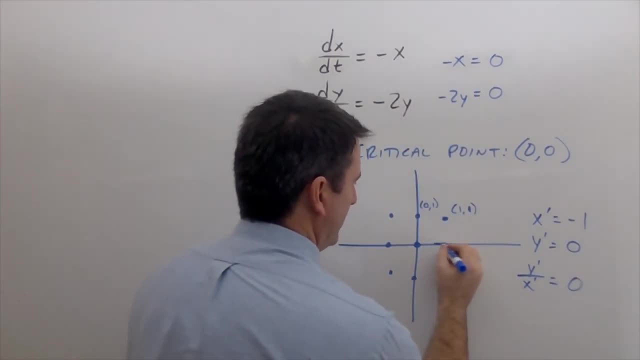 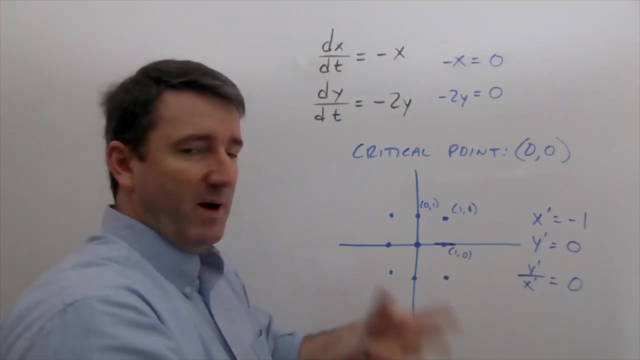 be zero. So, right here, at this point, our slope is zero. Now, which direction is it going? Well, if the change in x, if the derivative of x with respect to t is negative, then it's going to the left. If it's positive, it's going to the right. With the change in y, if it's positive, it's going. 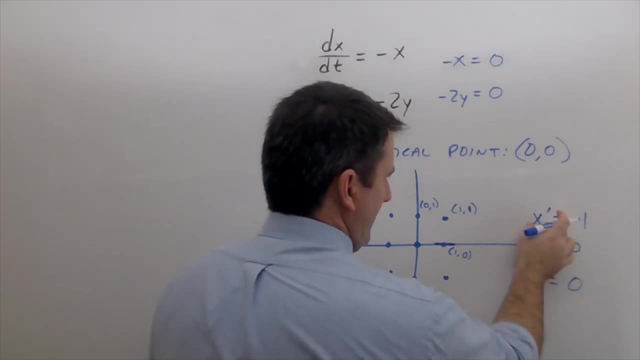 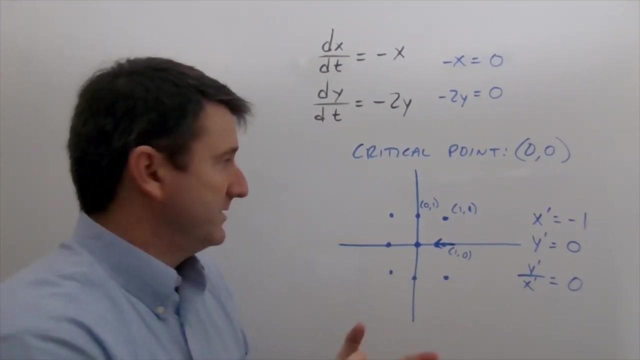 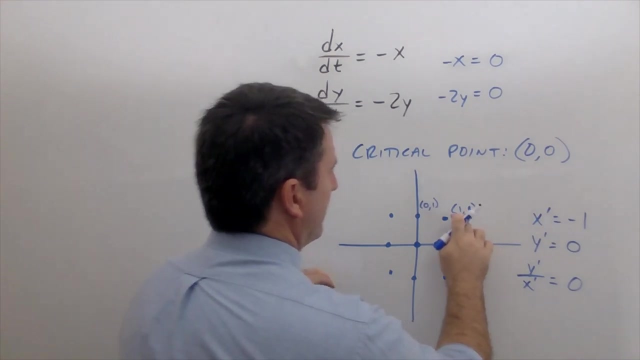 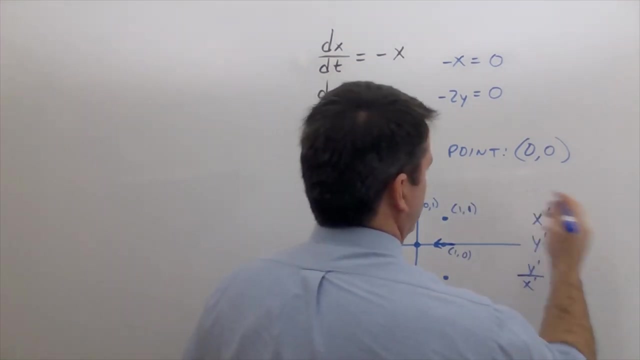 up. If it's negative, it's going down. So here the change in x is negative, so this is going to the left. So there's one of our arrows in our direction field. All right, now let's just work our way counterclockwise here. So if they're both 1, well, if x is 1, then the derivative of x. 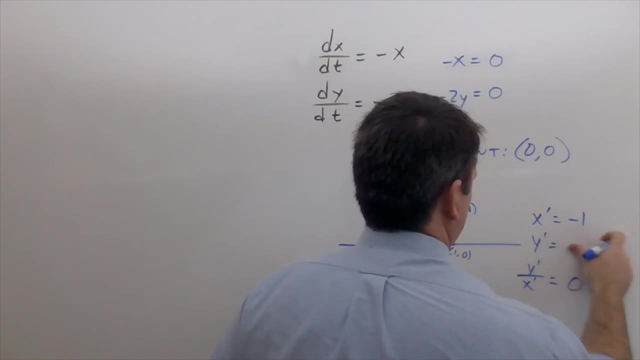 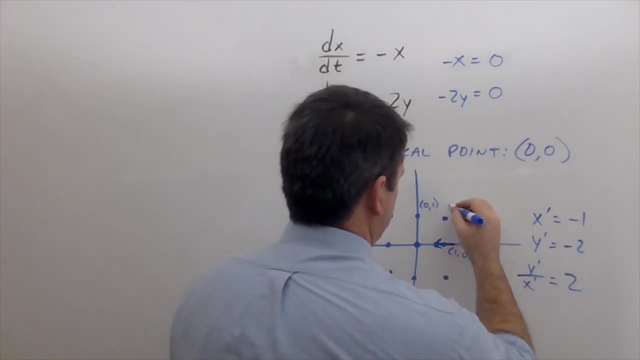 is going to be negative 1.. And if y is 1, then y prime is negative 2.. So the slope, the change in y over the change in x, is going to be 2.. So we're going to have a slope of 2 here And now, which direction is it going? 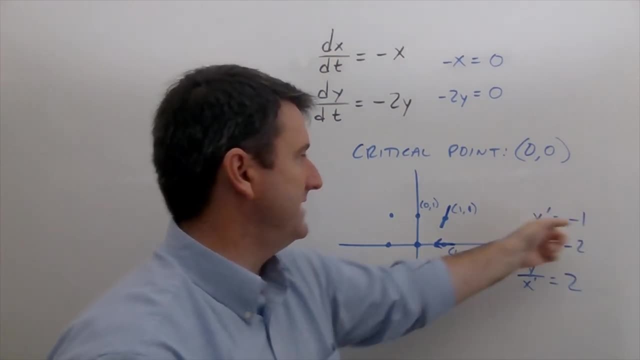 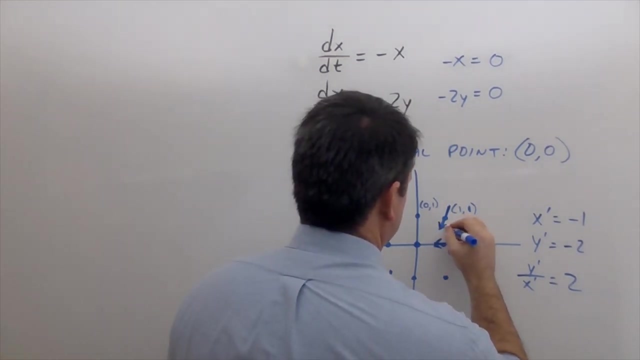 Well, the change in x is negative, so it's going to the left. The change in y is negative, so it's going down. So it's going down and to the left, So it's going this way. All right, now for the point. All right, well, x is 0, so the change in x is 0.. 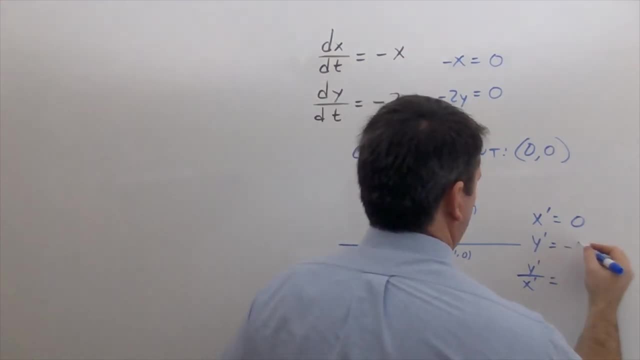 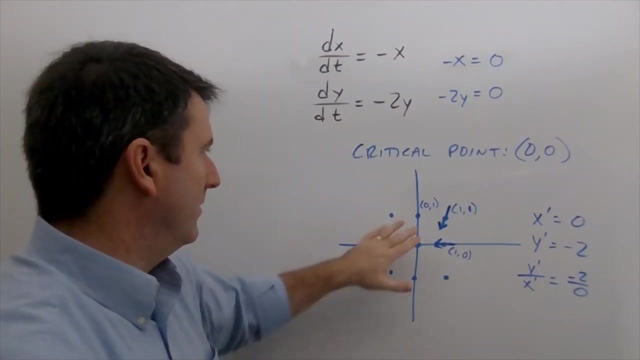 y is 1, so the change in y is negative 2.. The change in y over the change in x is negative: 2 over 0. That's a problem. So you can see that where x is equal to 0, we're not going. 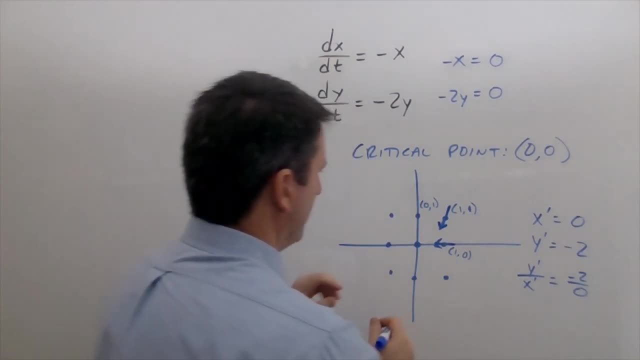 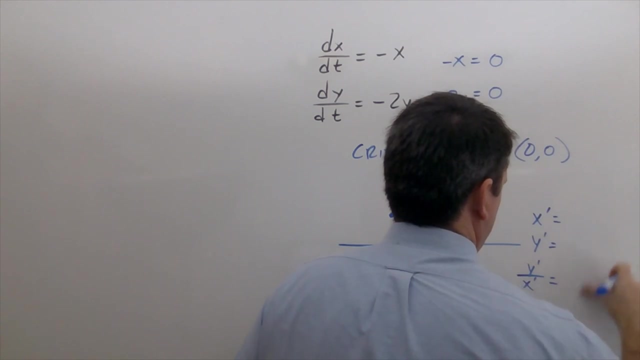 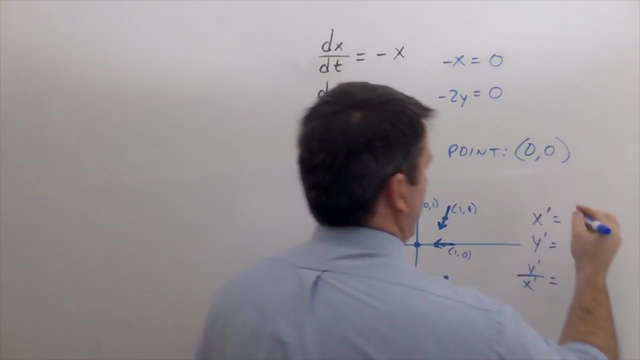 to have a trajectory. It's just not going to exist There on the y-axis here, So we won't draw an arrow there. Let's go over here to negative 1, 1.. Plug in negative 1 for x. We get 1 here. 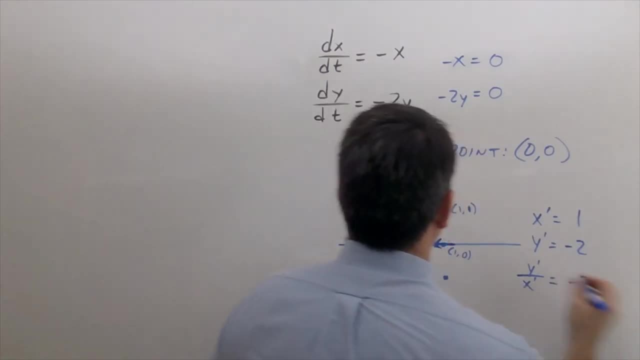 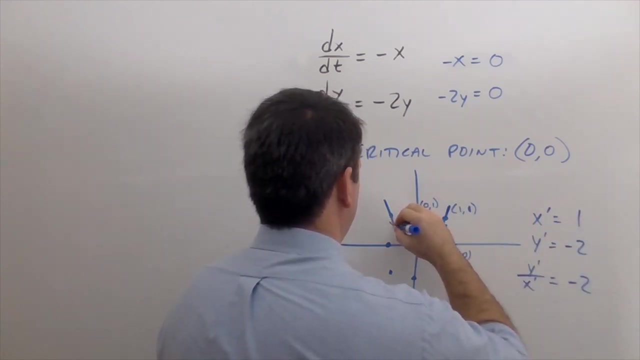 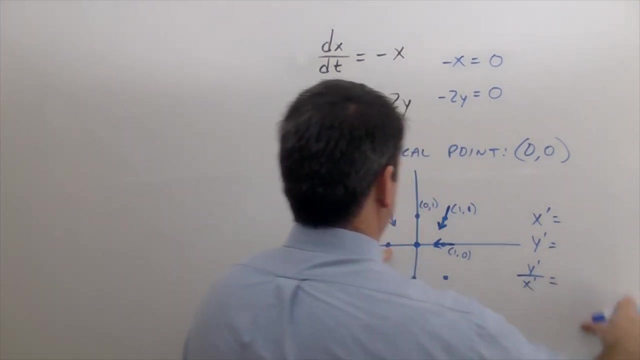 This is going to be negative 2.. So our slope is negative 2.. We'll draw our slope there. It's going to the right and down, So draw our arrow like that Here at the point. Well, we can see that if we plug in 0 for y. 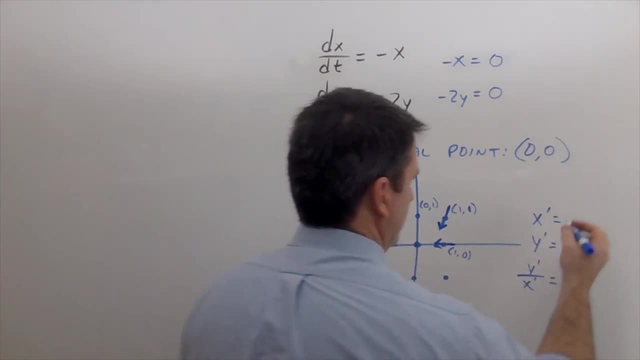 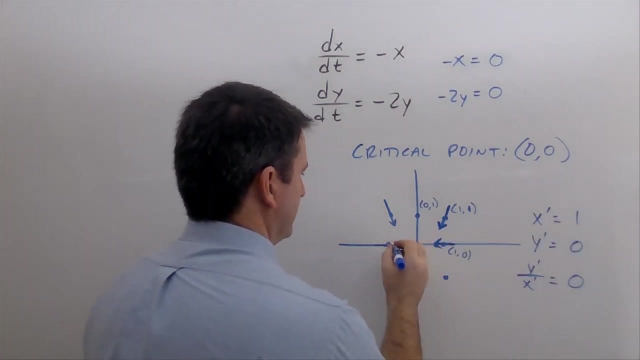 this whole thing is going to be 0. So our slope is 0.. Let's go ahead and write this in. This was the point. So this was 1 and 0.. Slope is 0.. It's going to the right because the change in x is. 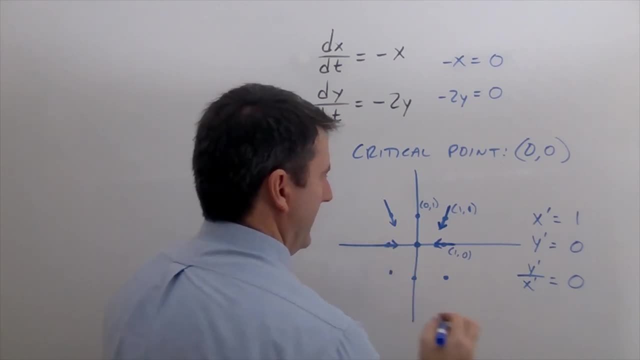 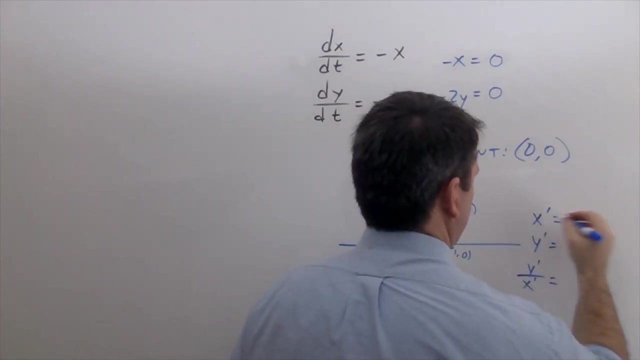 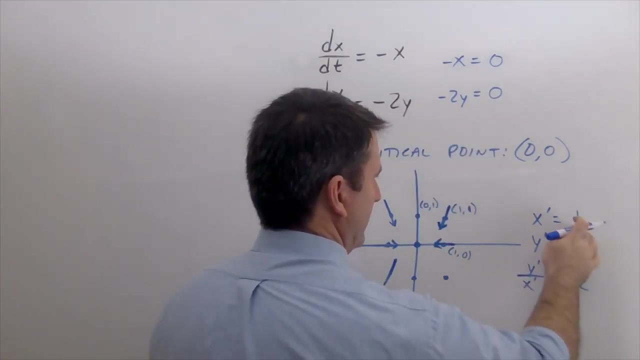 positive And then a couple more. This one negative 1, negative 1.. This is going to be 1 and 2.. So our slope will be 2.. We've got a slope that looks like that And it's going up and to the right. 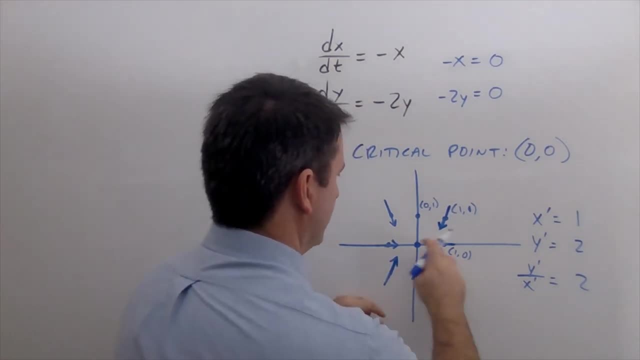 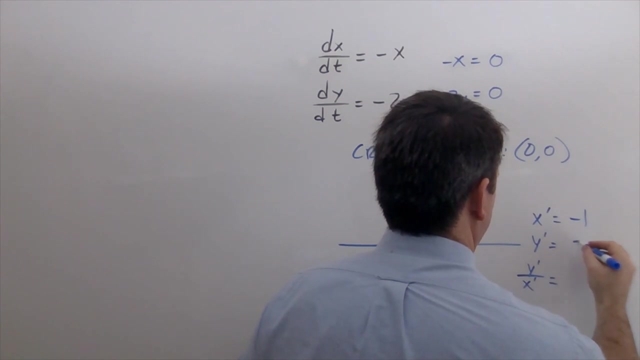 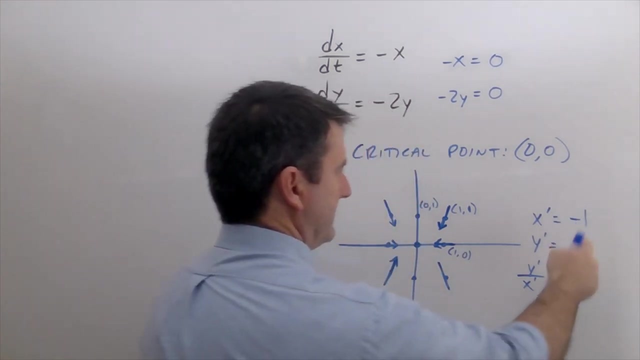 So our arrow looks like that, And then down here the point, We're going to get negative 1 and positive 2.. And that's going to give us a slope of negative 2, which looks like that, and it's going to the left and up. 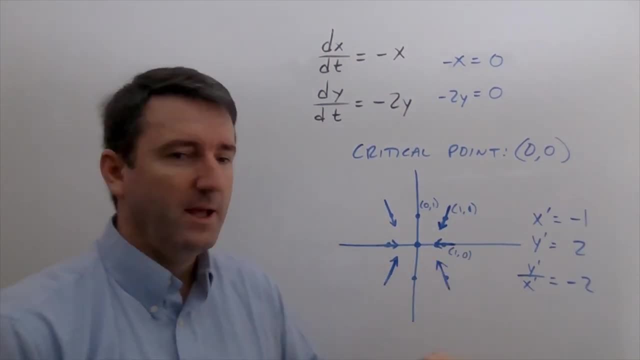 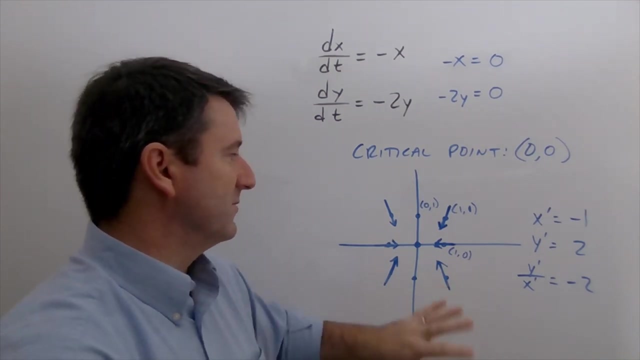 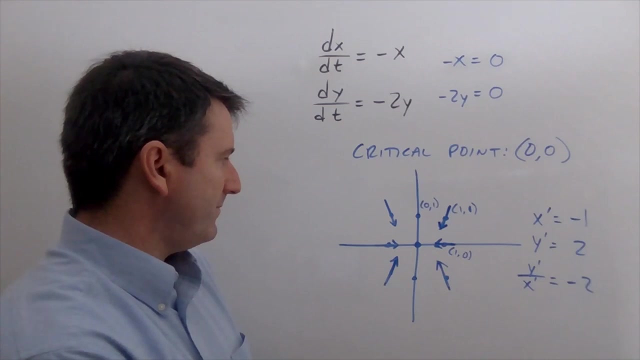 so our arrow looks like that. Alright now, obviously this gets tedious to do too much of this, so in future examples we're just going to turn to a computer and let it find our direction field for us. but you can see that with all of these, with 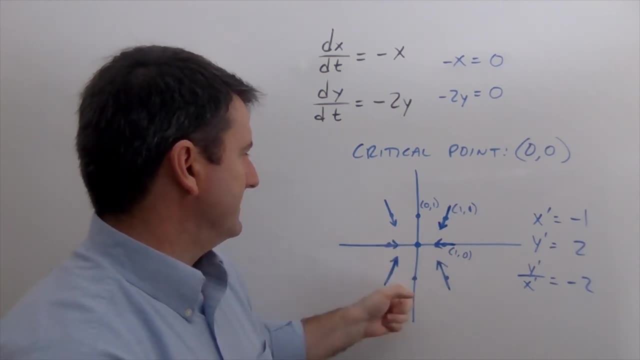 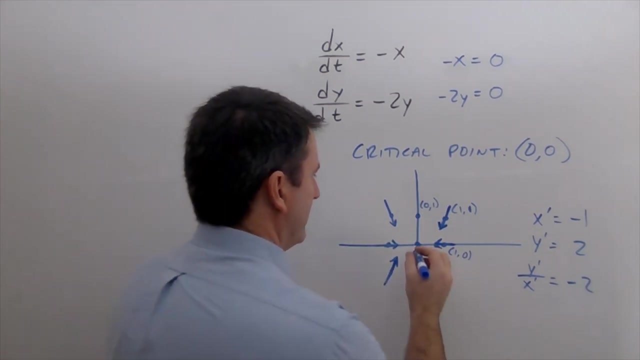 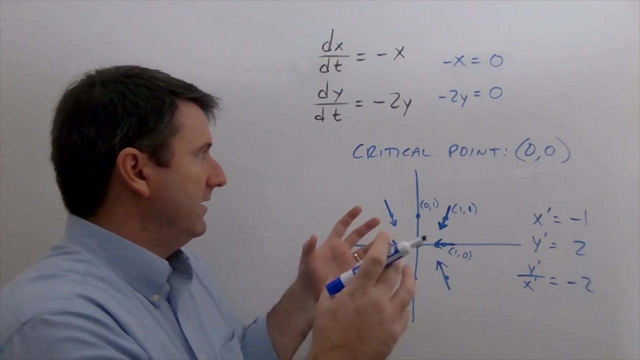 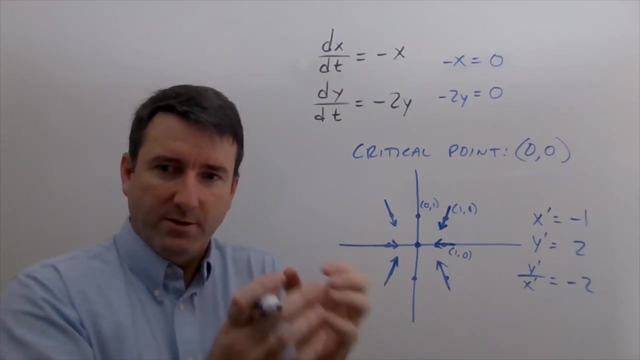 all of these trajectories here they're all. they're all bringing us to our, to our critical point. so our critical point here: if you can imagine, if you're on that critical point, obviously you're, you're not going anywhere, you're, there's no arrow with at the critical point, you're just stuck there. but what would 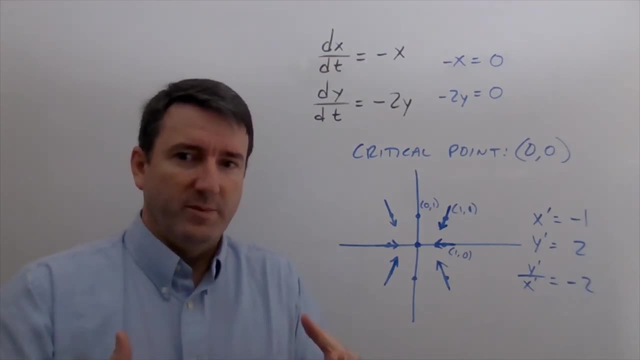 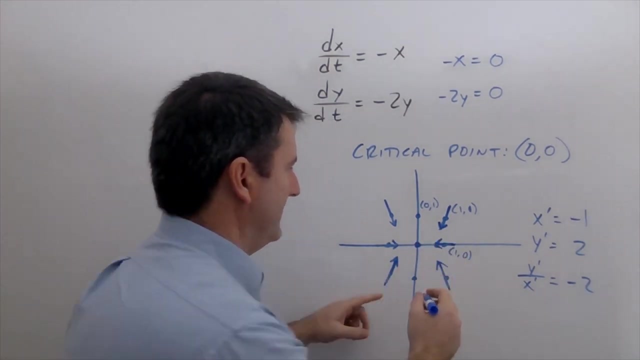 it. what would happen if you moved off of that critical point just a little bit? that's what's going to determine whether it's stable or unstable. so here, if you move the little ways off of this, well, it doesn't matter which direction you move. those trajectories are going to bring. 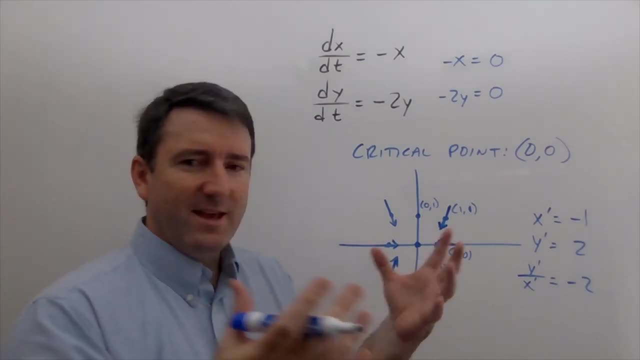 you right back down. I think of this as as like having a hole in golf at the, at the bottom of a bowl where I know, even if you miss by a little bit the, the bottom of a bowl where I know, even if you miss by a little bit, the- the. 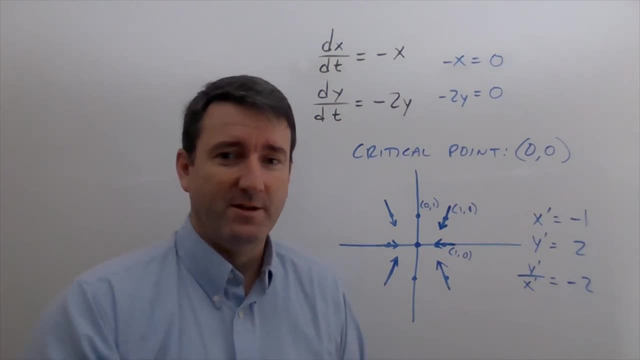 the slope is just going to bring you right back down to the, to the hole. you see those kinds of holes and in miniature golf, where you can, you can miss by quite a bit and it's still. everything is going to just funnel down into the hole. that's going to be a stable point. in fact it's going to be called 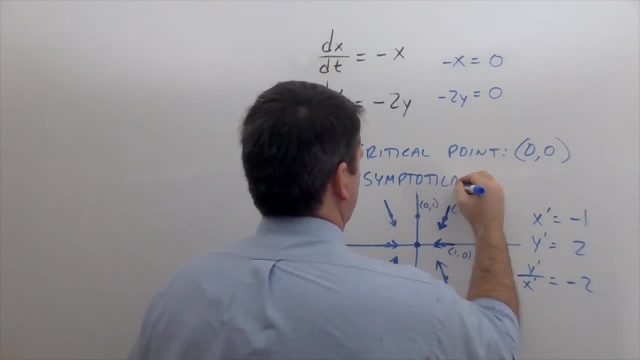 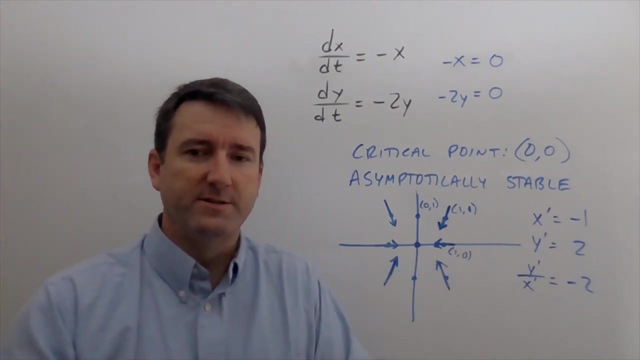 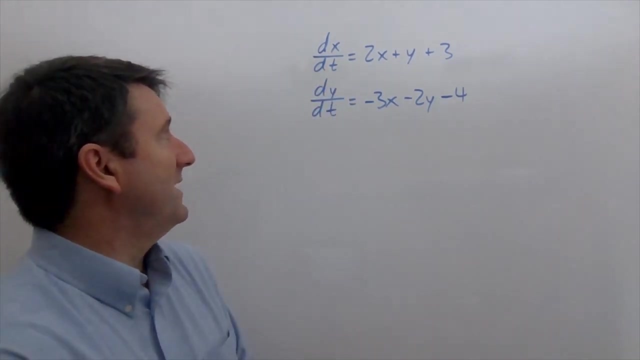 asymptotically. so we have this point where all the trajectories are going toward the critical point. we're going to call that asymptotically stable. So that's example number one. Alright, example two: we've got dx, dt equals 2x plus y plus 3 and dy. 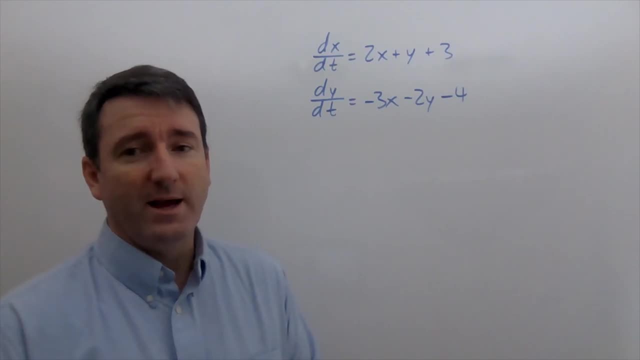 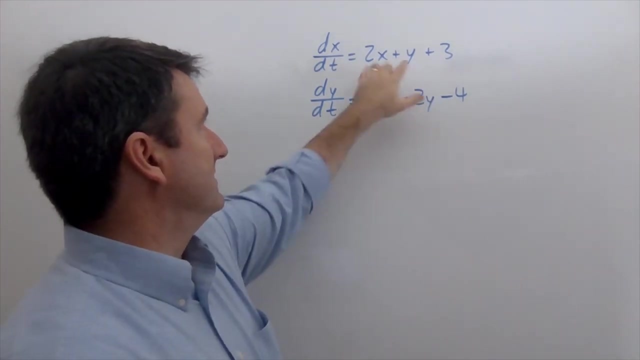 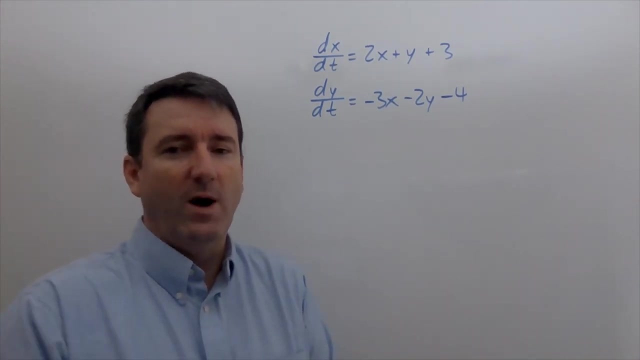 dt equals negative 3x minus 2y minus 4.. So to find the critical points for this, we're going to set each of these functions- this function here and this function here- equal to 0 and then figure out what for what values of x and y are. 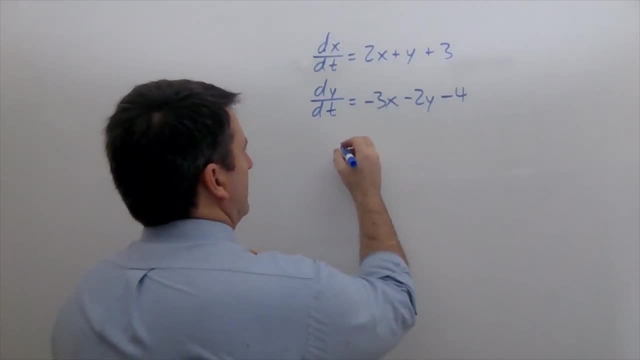 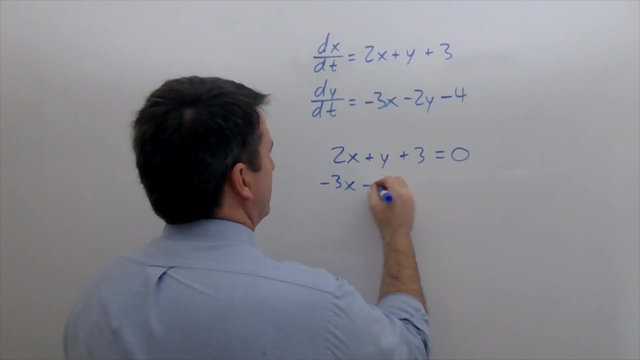 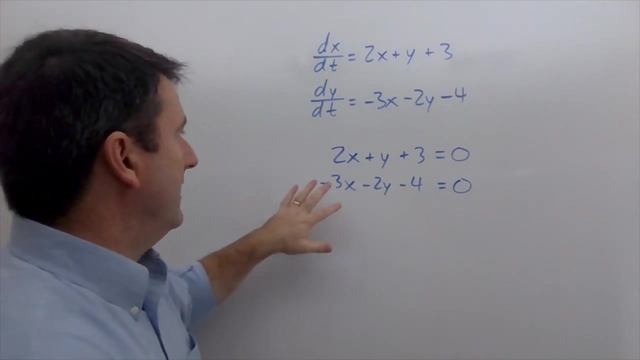 both of these going to be equal to 0.. So we've got: 2x plus y plus 3 is equal to 0, and negative 3x minus 2y minus 4 equals 0.. Alright, now to solve this system, let's. 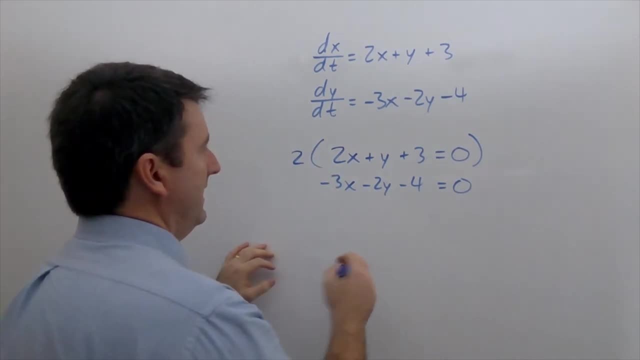 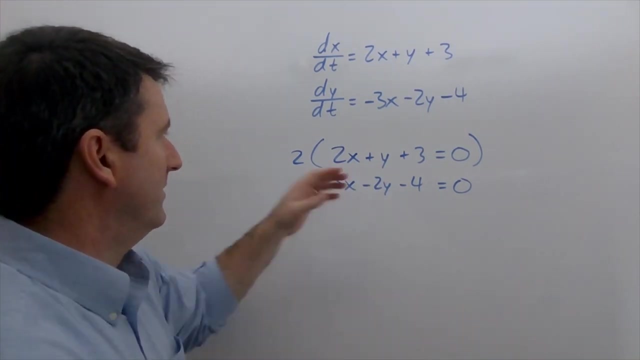 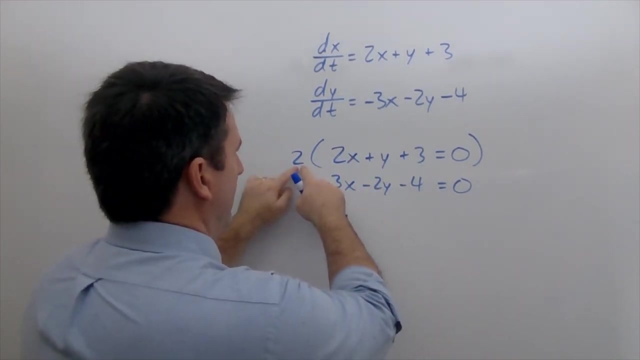 multiply this top equation by 2 and add it to our plot, the bottom, that will. that will give us 2y minus 2y, The y's will add to 0 and we'll be left with the x's. So 2 times 2x is 4x minus. 3x is x. 2 times 3 is 6 minus. 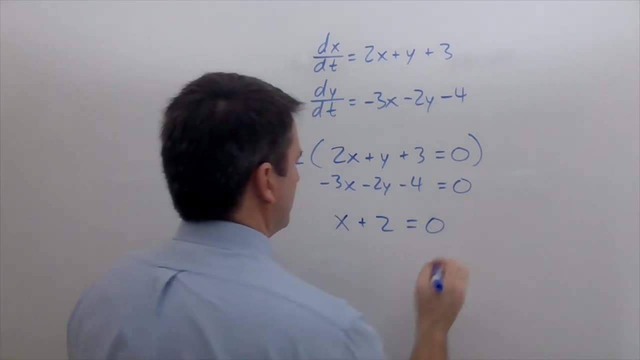 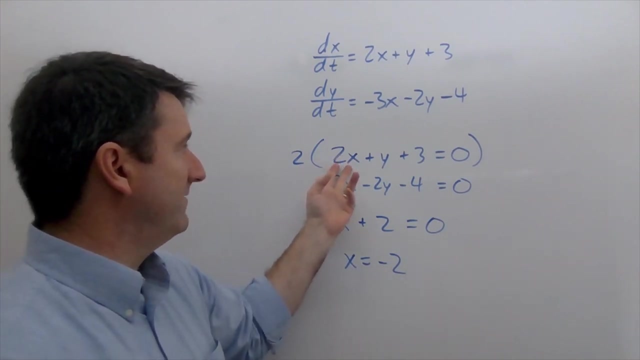 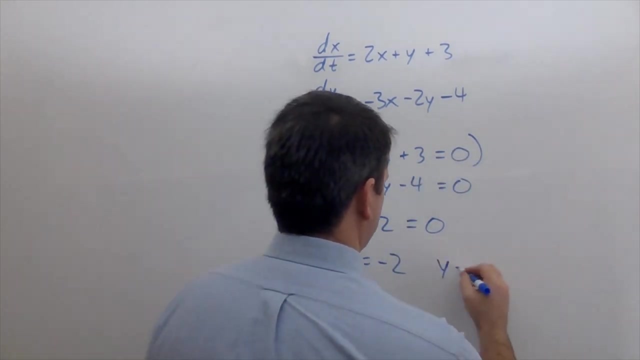 4 is 2.. So x plus 2 is 0, so x equals negative 2.. If we plug in negative 2 up here we get negative. 4 minus 3 is negative 1, so y minus 1 equals 0, so y is. 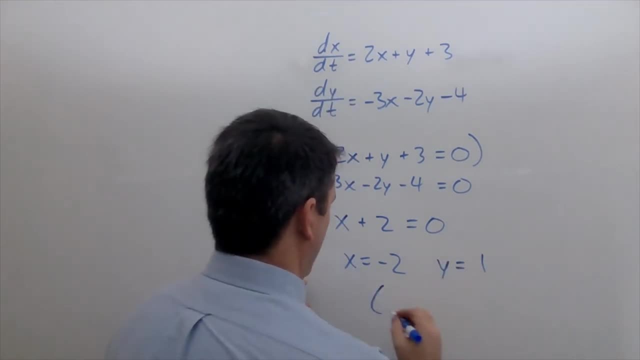 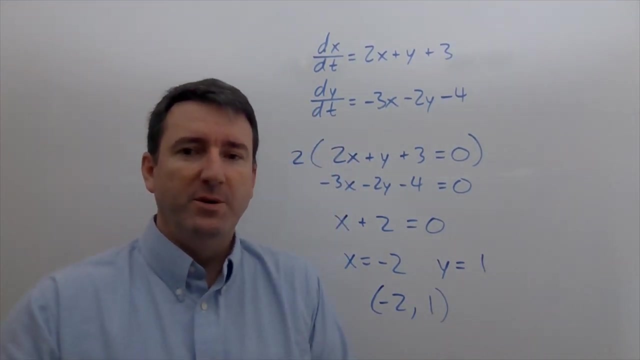 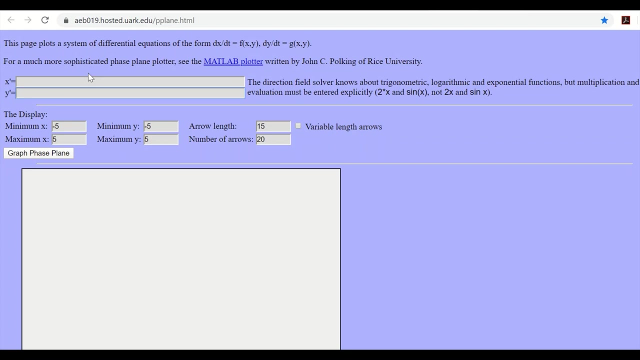 1.. And so our critical point is going to be at the point negative 2, 1.. All right, now let's go to the computer and sketch our direction field. All right, there are a number of phase plane plotters that you can find on the internet. 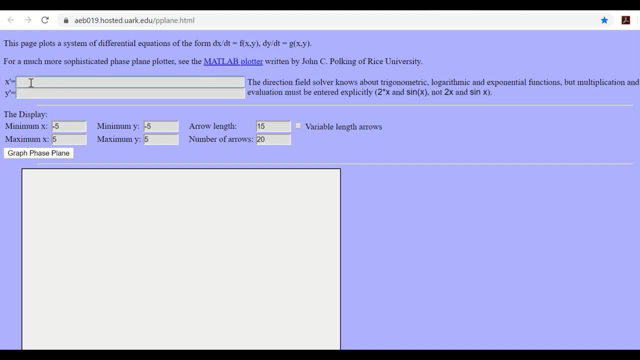 So let's go to the computer and sketch our direction field. All right, there are a number of phase plane plotters that you can find on the internet. I'm going to use this one that's on the University of Arkansas's website. So 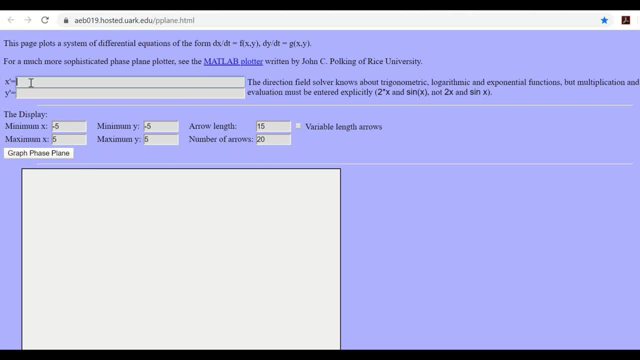 we're going to first enter x prime, which is was equal to 2 times x plus y plus 3, and then y prime was negative: 3 times x minus 2 times y minus 4.. And let's go ahead and graph that phase plane and there you can see that 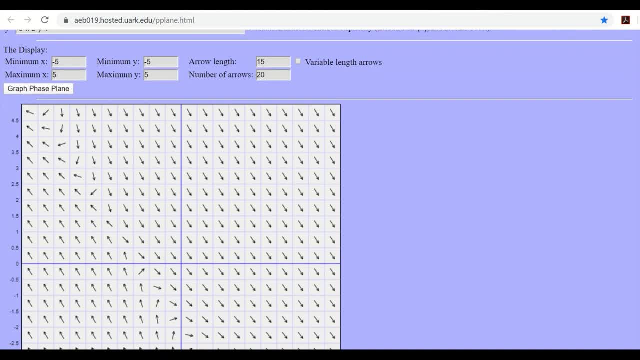 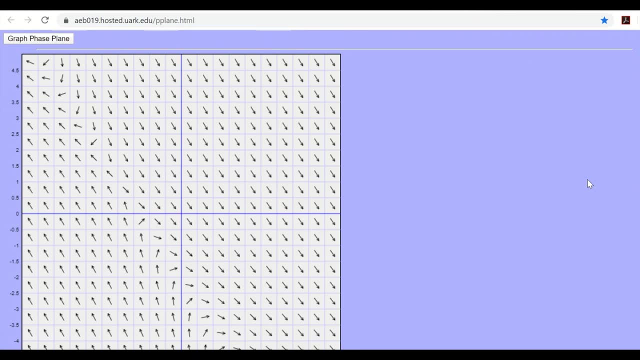 very quickly we get, we get a graph of this phase plane And what we're looking for is our critical point, which we determined earlier was going to be at the point negative 2, 1.. So if we go out to negative 2 right here and then up to 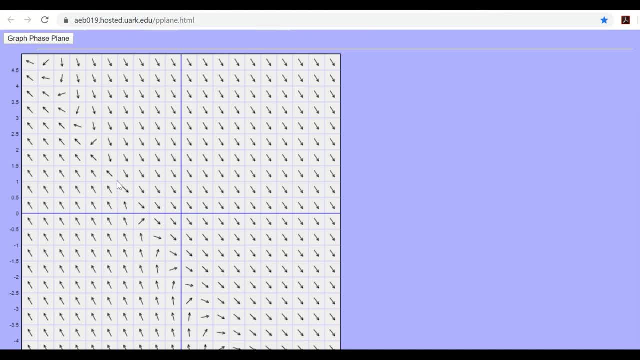 1: here's our critical point, right here, And if we graph right around that point, if we, if we just look at what happens, if you've got a something right in around that point, what happens to it, and so we're going to graph a bunch of these different solutions, starting in